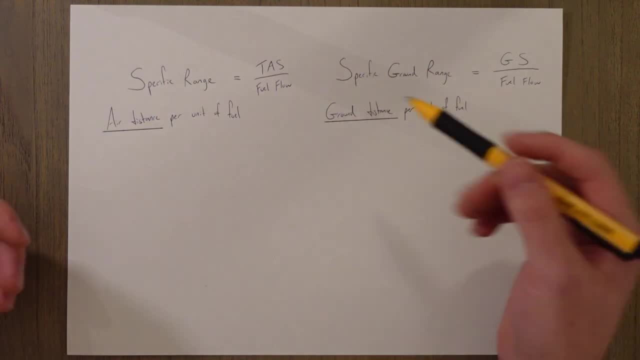 our specific ground range will be the same. The units for specific range will be nautical miles per kilogram of fuel used. The units for specific range will be nautical miles per kilogram of fuel used, and if we divide by time, we can get two formulas, one for specific range and one. 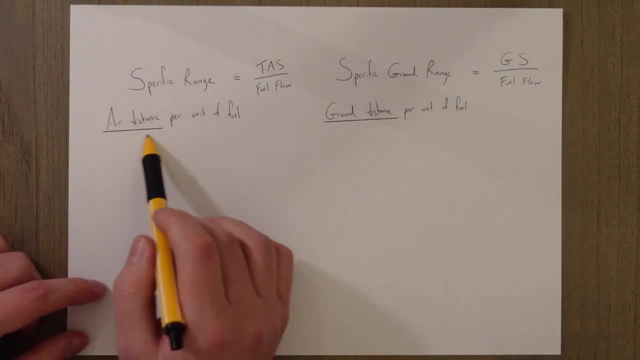 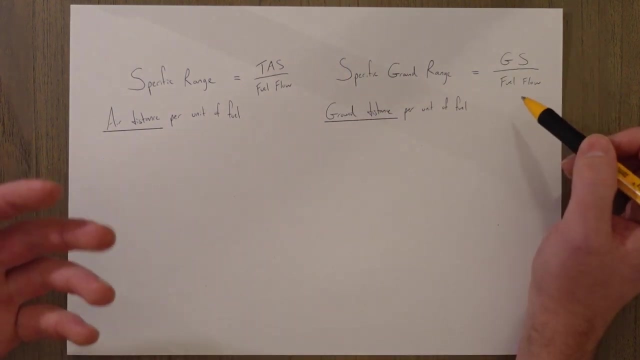 for specific ground range. the one for a specific range, the air distance would be the true airspeed over fuel flow, and for ground range we just need to factor in wind, and we can do that by using the ground speed, which is the TAS, plus or minus any wind component, and then divide that by the fuel flow as well, depending. 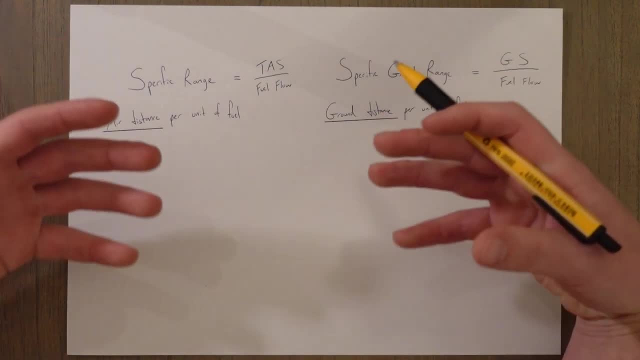 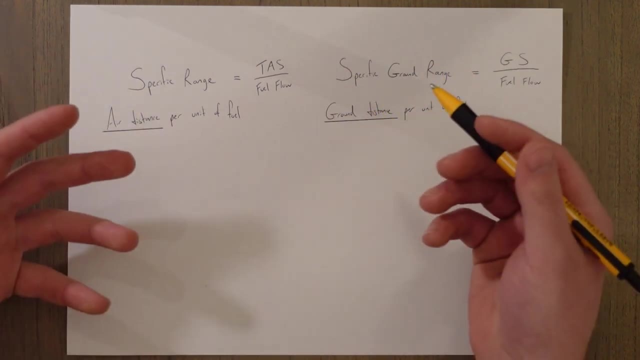 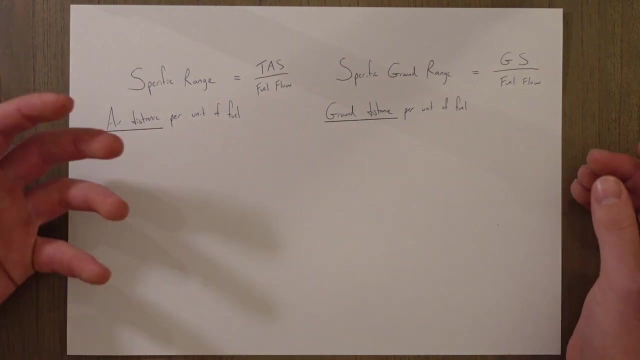 on the conditions we are flying in. we need a certain amount of thrust that we need to overcome all of the thrust required or the drag that is produced when we fly. thrust generation requires us to use up fuel, and how much fuel depends on the specific fuel consumption of the engine. this is basically a 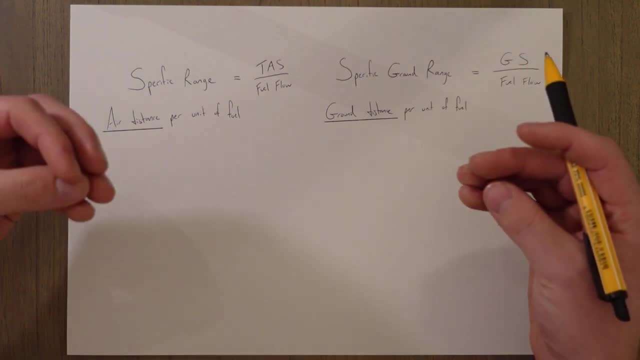 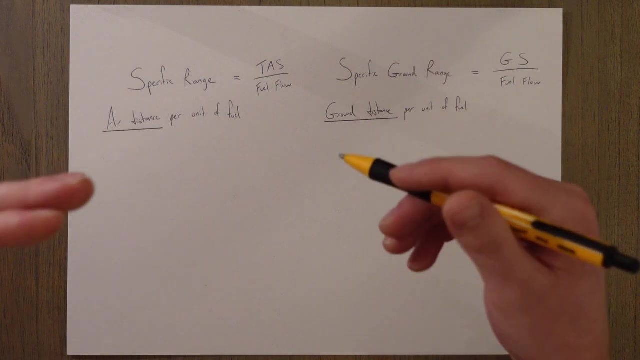 measure of engine efficiency, and it is the amount of fuel flow needed to produce one unit of thrust. in a jet aircraft and a propeller, it's the amount of fuel used to produce one unit of thrust of power. why is this important, though? well, we already have a formula for. 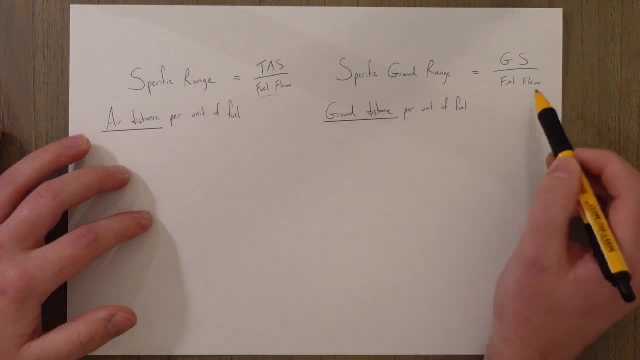 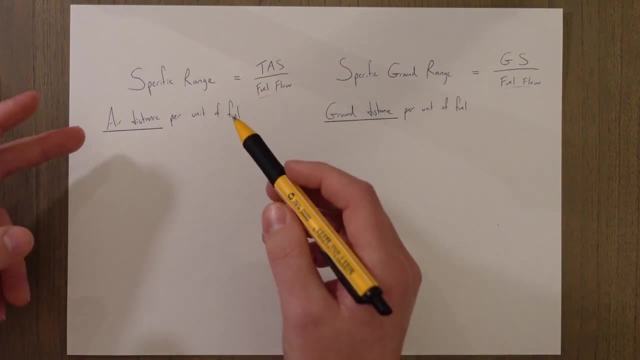 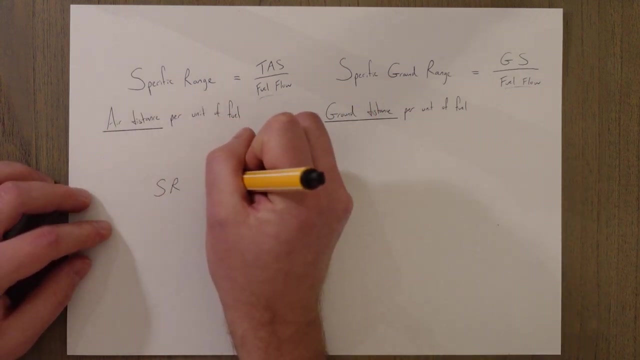 specific range and specific ground range. but we can break down the fuel flow into a little bit more detail. if we first have a look at the jet aircraft then we can substitute in the value for specific fuel consumption into the specific range equation and get specific range is equal to the true airspeed over the specific 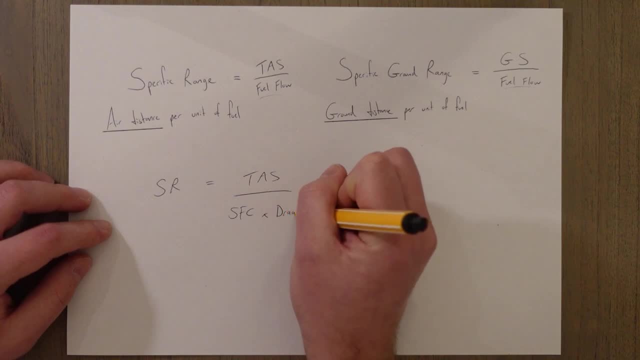 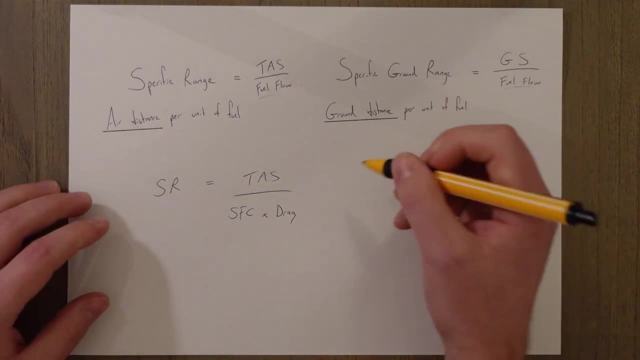 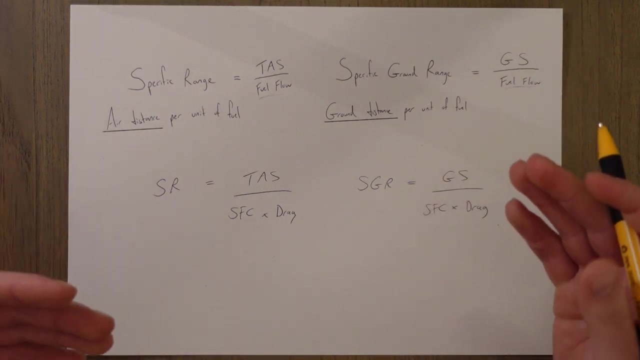 fuel consumption, times, drag or the amount of thrust required for that phase of flight. or if we want to find the specific ground range, we just have to substitute in ground speed for a propeller. it is slightly different. the difference is that bottom line where we have to have the consideration of specific fuel consumption. 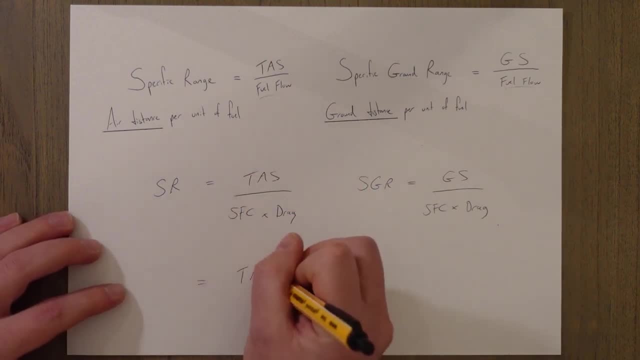 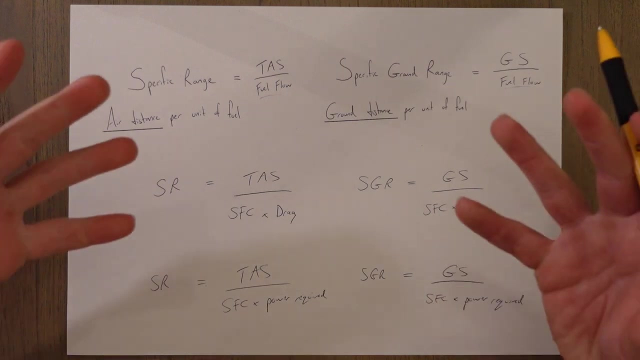 per unit of power. so we get the same equations, but on the bottom line it's power required at that phase of flight. so how have we substituted in those values for, instead of, fuel flow? basically? well, it basically allows us to see a bit more clearly the factors that affect fuel flow and our specific range. so 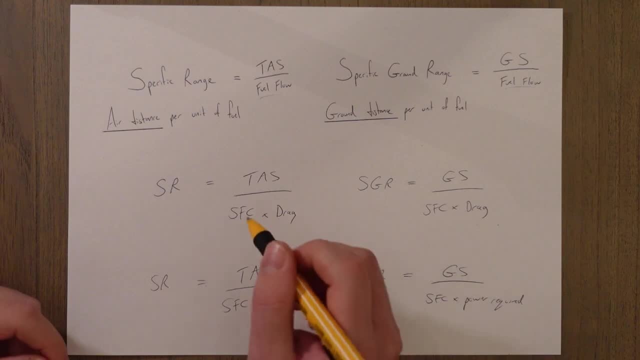 if we look at this one, for example, we know that if the specific fuel consumption is high and the drag is high, that means that we're going to be dividing by a larger number and that means our specific range is going to go down. if we take the specific ground range of the propeller, for instance, 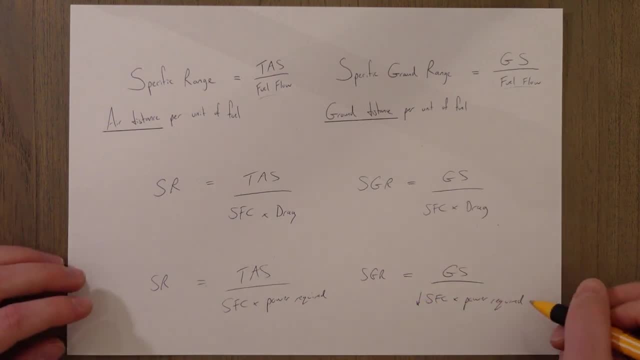 if we have a low specific fuel consumption and a low amount of power required, we're divided by a small number, which means our ground range is going to be high. it's just an easy way to analyze. range is influenced according to a number of factors. most of them you can figure out by looking at. 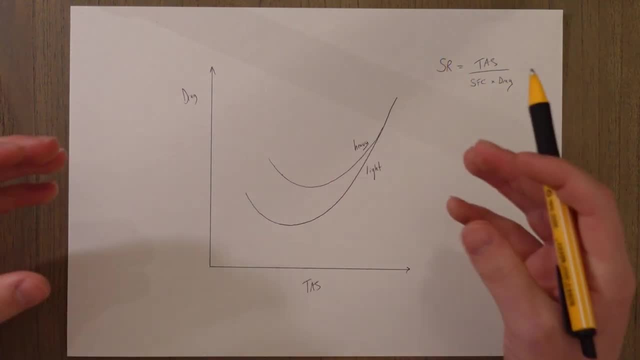 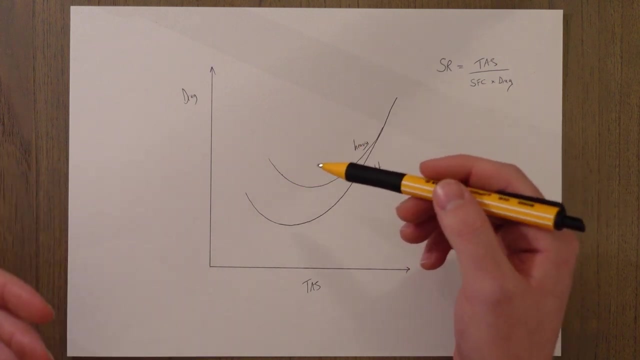 the equations that we've just worked out. but first we're going to have a look at mass. if we compare a light aircraft to a heavy one, the total drag curves look like this: mainly because they produce more lift, a more induced drag is generated. result: this means that on the lighter 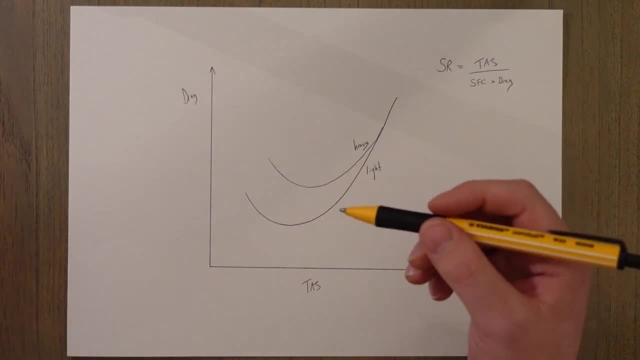 aircraft, the drag is lower when we fly at the speed for Max range, which, now that I think about it, I've not actually talked about the speed for Max range, so let's just do a little sidebar here. so Max range is called VMR or, if you're flying at Mac numbers, MMR, speed, Mac number- and it occurs. where, if you're flying at a maximum speed, you're going to have a slow drag and then you get a speed. so the speed that I'm going to use for Max range and if you're flying at a maximum speed, you're going to speed and it occurs where the speed that we have it's going to be the speed that we're going to you're. 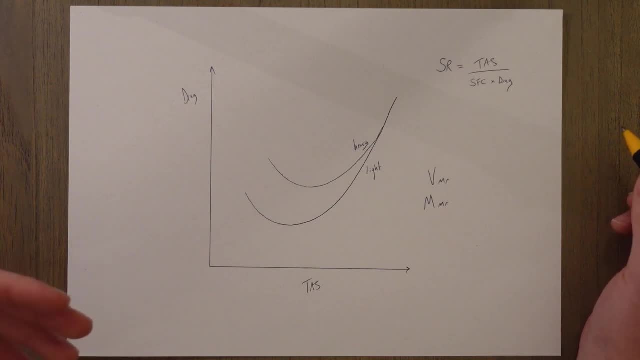 we maximize our thrust to drag ratio and in a turbojet or a jet in general, this occurs at 1.32 VMD and this is the tangent on this curve. so if you go something like that, this value here is our VMR, which will be 1.32 VMD In a 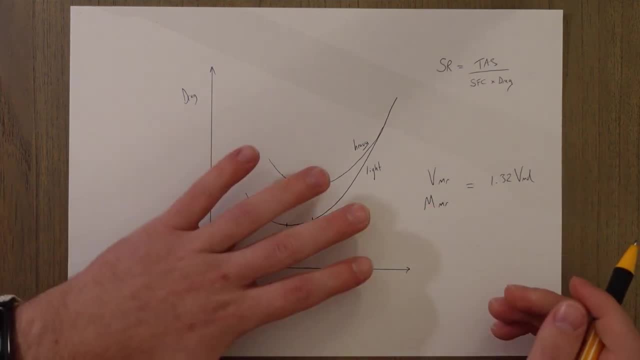 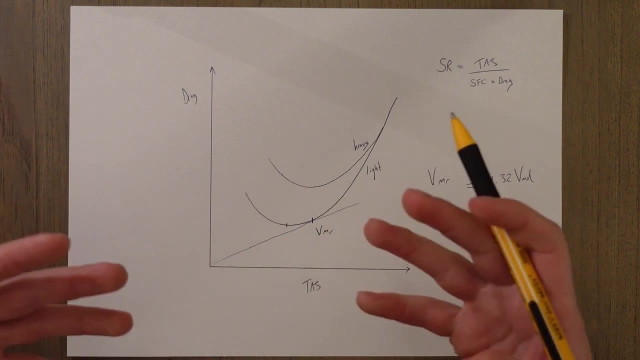 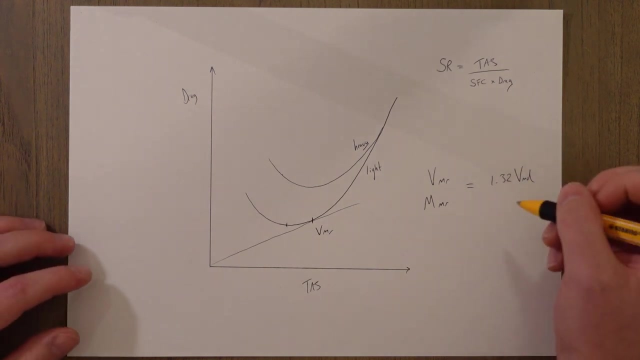 propeller driven aircraft. we take the tangent to the power curve, not this drag curve, and it's the same effect. we're maximizing our thrust to drag or thrust to power required ratio and this actually occurs. therefore, a 1.32 VMP speed for minimum power which, coincidentally, is actually VMD, because 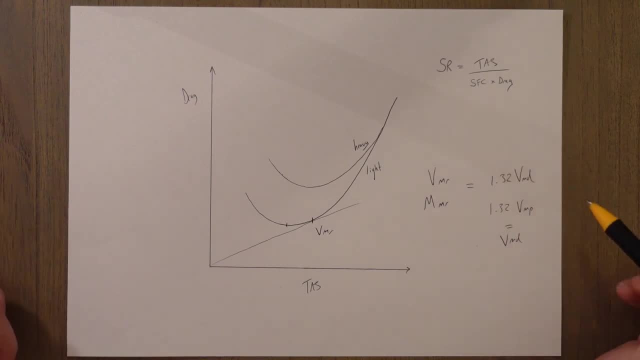 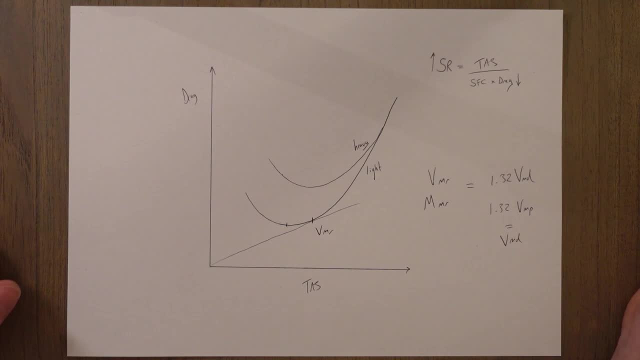 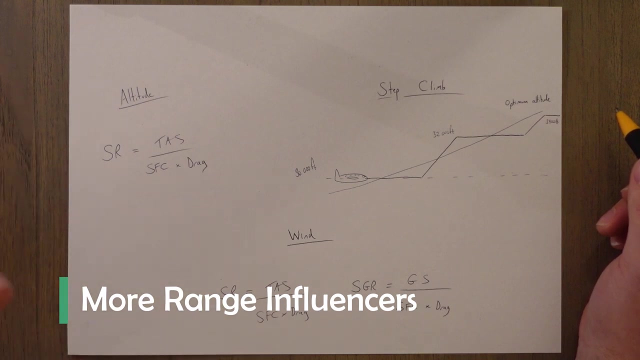 number, which means your specific range, goes up. simple as that. and also take note that if we are lighter, our speed for VMR would be a bit slower as well. so that would be VMR in the heavy aircraft, and then, as we get lighter, our speed slows down. same for the propellers if an aircraft is flying at its optimum. altitude, the rate of acceleration is a bit slower than the rate of acceleration range will be maximized. This optimum altitude in a turbojet is high up. Basically the engines are running at their designed rpm because they're designed to cruise, because that's where they spend. 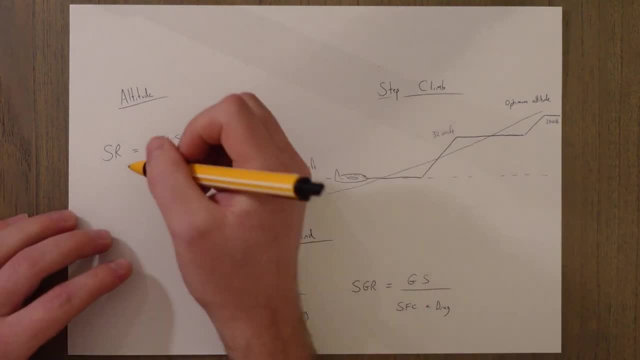 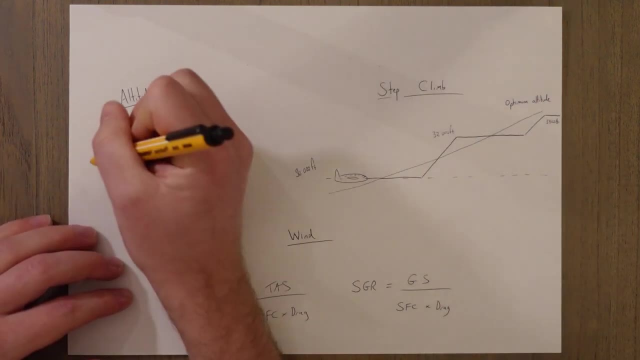 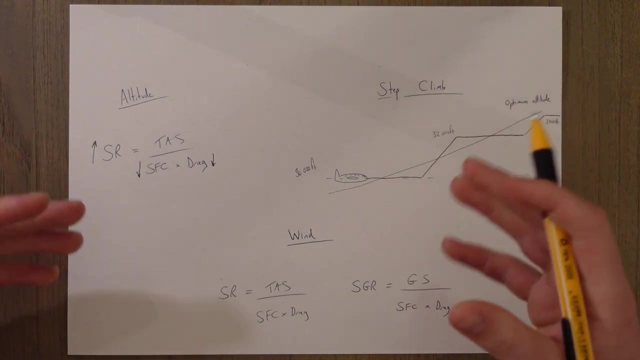 most of their time and that's where they are most efficient, making the specific fuel consumption low. and also up at altitude the air is less dense, meaning drag is lower, so our specific range goes up, and our specific ground range would go up as well. In a propeller driven aircraft, the optimum 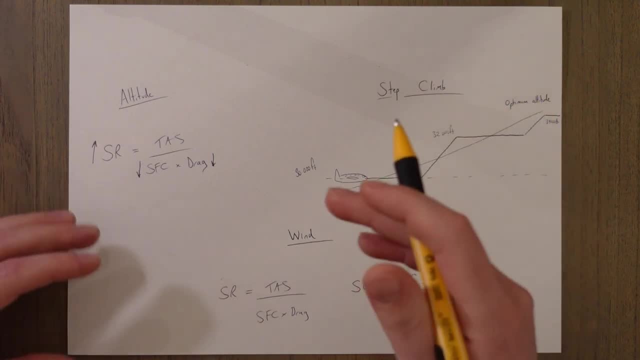 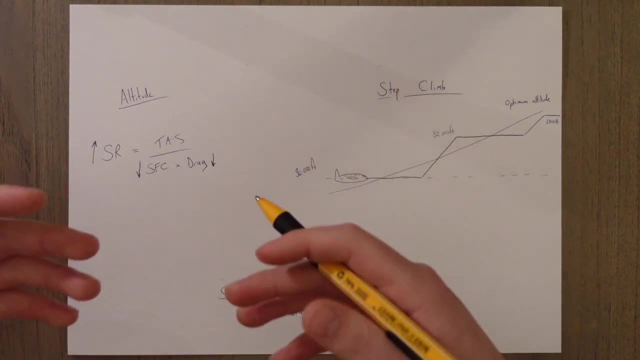 altitude isn't as simple, as it depends on throttle position and propeller rpm combinations and optimum combinations and altitudes are often tested out and put in manufacturer's manuals, so it's hard to say. but it's not going to be quite as high up. it's going to be the position for. 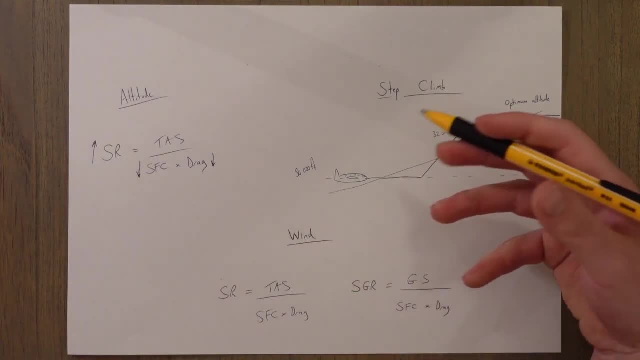 basically maximum throttle open. So altitude and mass are the two biggest influencers on commercial aircraft. The optimum altitude is not as high up as it's going to be for maximum flights, so this is an example of a step climb. it's something you see quite often. So say we. 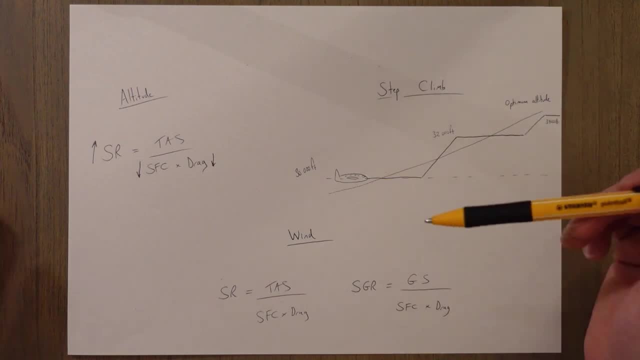 first reach our cruising altitude of thirty thousand feet. we're heavy and full of fuel, and as we cruise along we burn fuel and weight. as a result. This means our drag reduces because we're needing less lift and therefore the specific range increases, which is good. we're. lowering our drag specific range goes up. This reduction in drag and a lower speed for maximum range requires less thrust to be used, so the engines don't have to work as hard, so the rpm of the engine of the route can reduce. This means that the engine may no longer be. operating in its ideal range, which is typically around ninety to ninety five percent. So we counterintuitively want to make the engines work a bit harder again to get them back into this efficient range range. We do this by climbing into less dense air, meaning more air has to pass through. the engine in order to generate the correct amount of thrust, and the engine has to rotate faster as a result, pushing us back up into the ideal RPM range. This means that, throughout the flight, our optimum altitude to keep the engines working in the efficient 90-95% range. 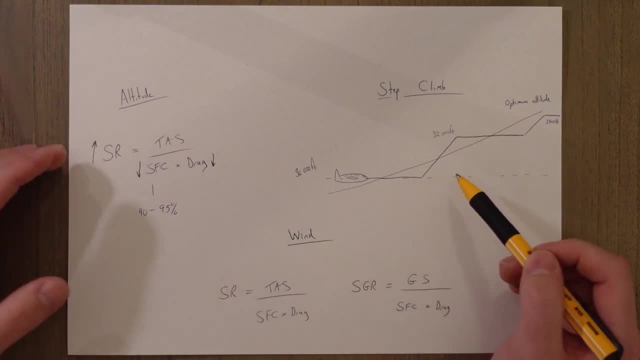 steadily climbs as we go throughout the flight, as we burn weight. In practice, though, we can't slowly climb along as we fly, because if everyone was doing it, there'd be a ridiculous number of collisions in the air. So what we do is we fly at one altitude: 30,000 feet. 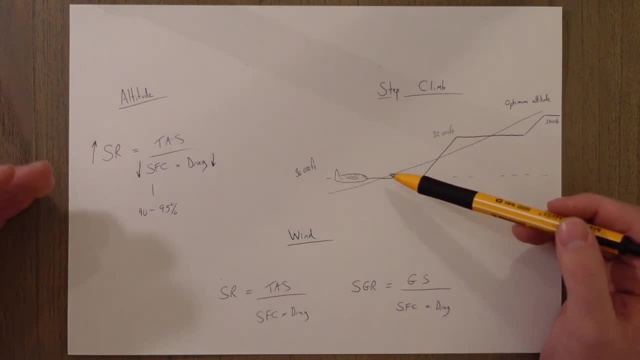 at the start, maybe slightly above the optimum altitude. then, as we burn fuel, the optimum altitude will climb up to meet us, then pass through our level Once it reaches 1,000 feet or so above. we would request to climb up to the next level, 32,000 feet. then again, 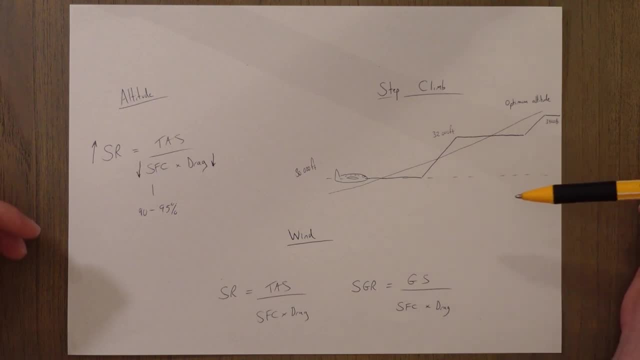 it would climb up to reach us, and so on and so forth throughout the flight Until we reach the structural limit of the aircraft. This is known as a step climb, and it's something you do almost every flight when you're flying commercially, just to save. 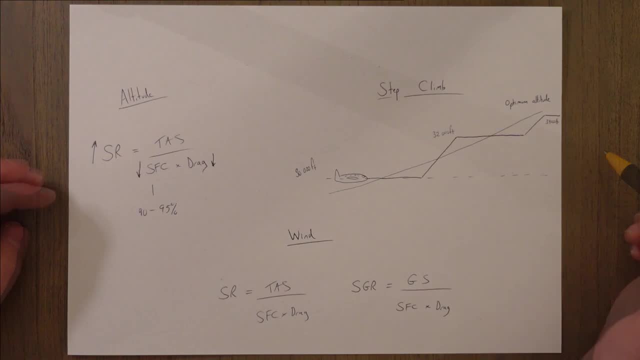 fuel by flying as close to the optimum altitude as possible. So wind influences the specific ground range, but not the specific air range. The specific range is the specific air range, but it's just called specific range. So basically it's because TAS and ground speed, while TAS is a specific air range, it's also a specific 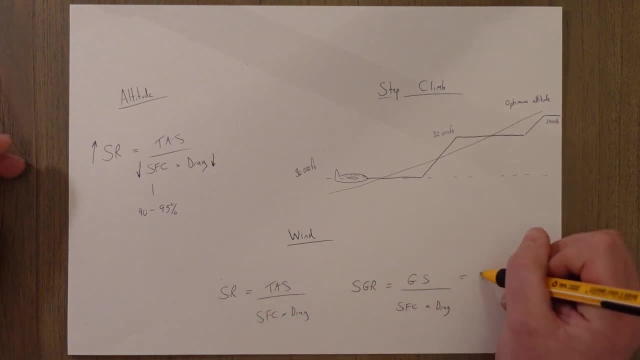 air range. TAS isn't affected by wind and ground speed is equal to TAS, plus or minus, whatever wind component you've got. So obviously the wind has an influence on this specific ground range, but nothing to do with the specific air range. So if we had a tailwind, our ground speed goes up and our specific range wouldn't change, but the specific ground change would go down as a result. Wait, did I say tailwind? If it's a tailwind, it would go up. If it's a headwind, the specific ground range would go down. 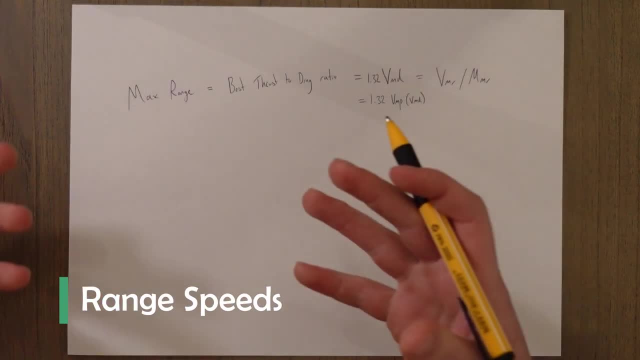 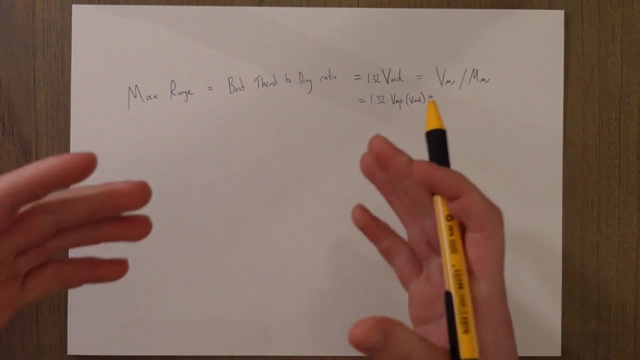 So that's how we get our maximum range out of an aircraft, but it does require us to fly at MMR or VMR, which might be a bit slow to get to our destination on time, to pick up more passengers or pick up some cargo, et cetera. So there's a commercial element. 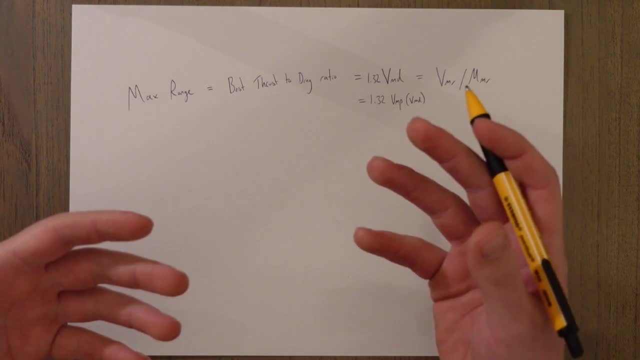 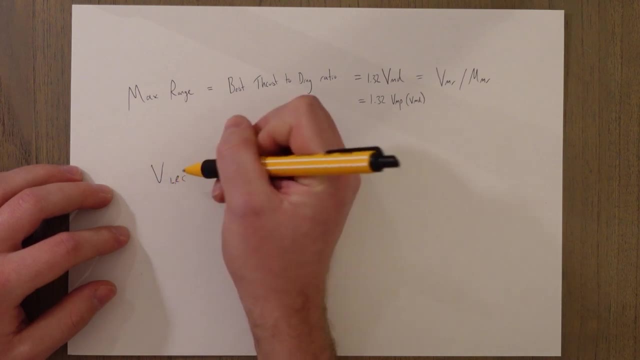 we need to think about. For this, there's a speed generated for using during the long range cruise, and it's called VLRC. This is a speed that's slightly faster. It's faster than the speed for max range, So there is going to be a bit more fuel burn. 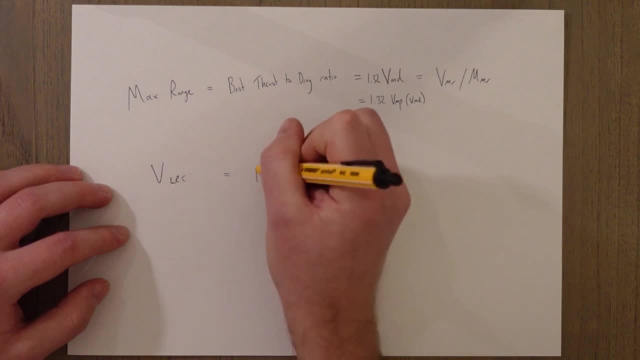 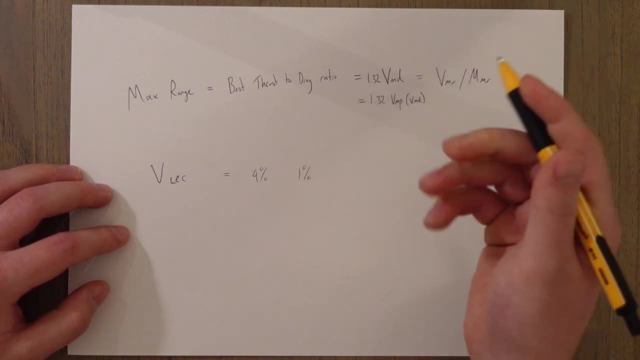 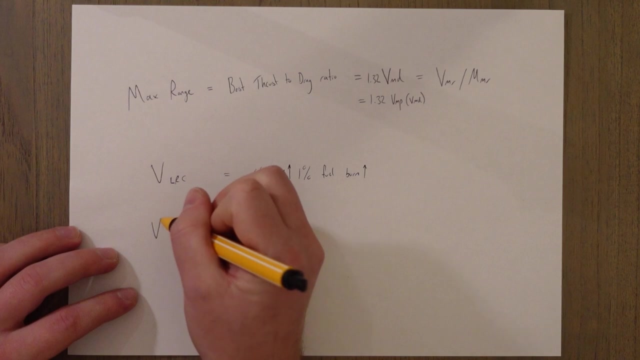 but it's calculated so that you get about 4% speed increase with about 1% fuel burn reduction or reduction range, fuel burn increase. And companies use this as a bit of a trade off. And there's also a speed which is called V econ. To be honest, they're very rarely. 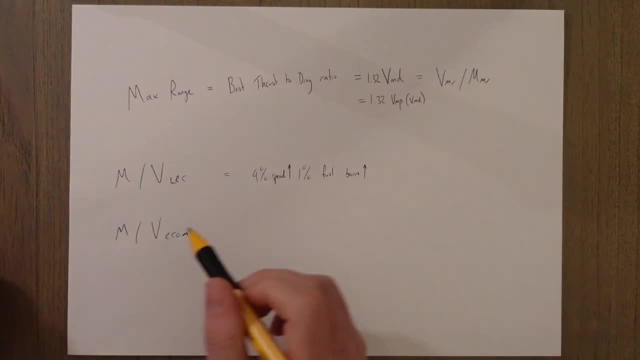 going to be V speeds, They're going to be max speeds, And the way we figure out the speed is by using the cost index. The cost index, which I talked about briefly in the class before, is usually in a range between 1 and 50, at least from what I've seen. anyway, You could get higher. I don't know- Boeing and Airbus both use it, but I'm not sure about other manufacturers- And it's basically a trade off between speed of flight and amount of fuel burn. If you have a really low cost index, you'd save a lot of fuel. but fly really. 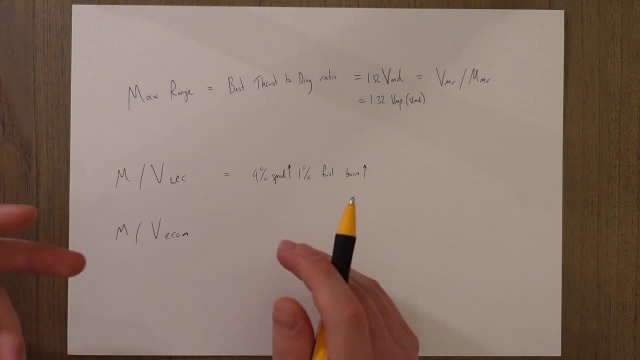 slow And a high cost index would be the reverse: fast flight burning lots of fuel. We're given this cost index by the flight planning department depending on how fast they need us to fly to arrive on time according to some timetables or slots or something like that at airports. 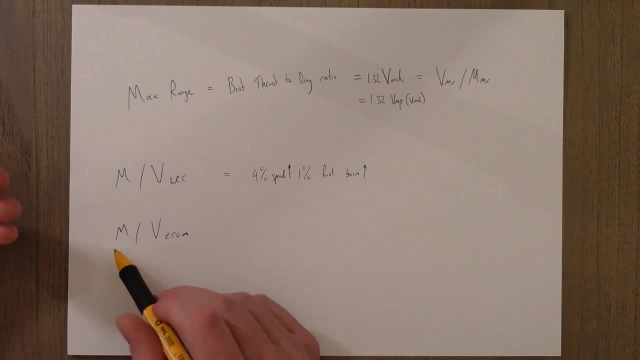 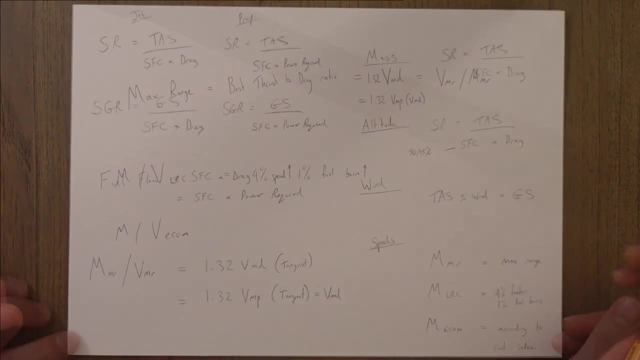 We then pop it into a computer on the aircraft and a Mach number for econ. in the cruise Our econ speed is generated and that's what we fly through the flight. Okay, So a specific air range or just specific range is the true air speed divided by the. 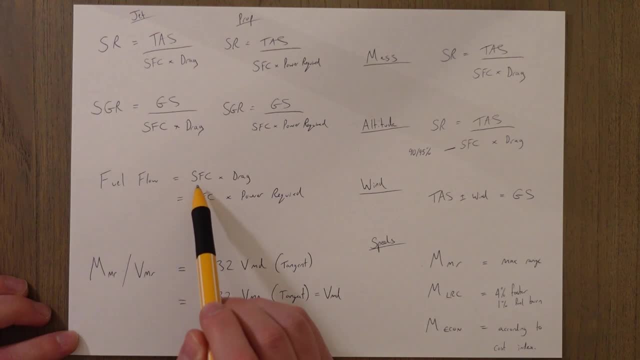 fuel flow And the fuel flow is specific fuel consumption times. drag for a jet And for a propeller. it is specific fuel consumption times, power required. Think of drag as thrust required. Maybe that might help. And if you want to convert them into specific ground range, you just need to factor in the 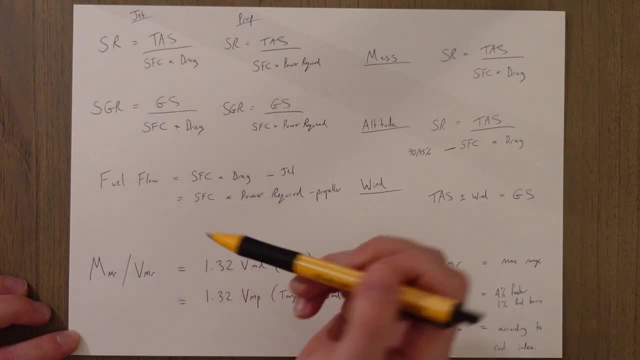 wind, And to do that you just convert the TAS into a ground speed, because ground speed equals TAS plus or minus N, Any wind component that's helping you. The speeds for max range speed MMR is going to be 1.32 times VMD. That's basically the. 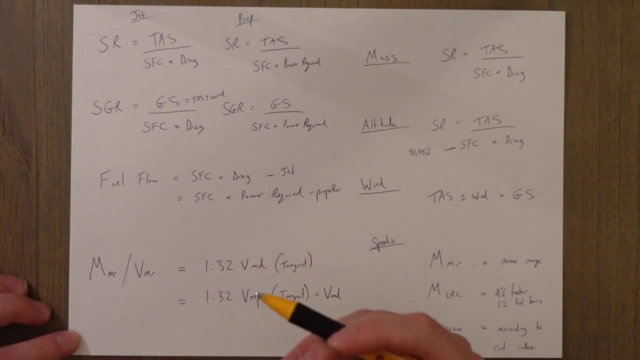 tangent to the drag curve, where our thrust to drag ratio is maximized. In a propeller it's slightly different. It's tangent to the power required graph And the tangent means that our ratio of thrust to power required Is maximized. And that occurs at 1.32 VMP which, just because of the maths, happens to.